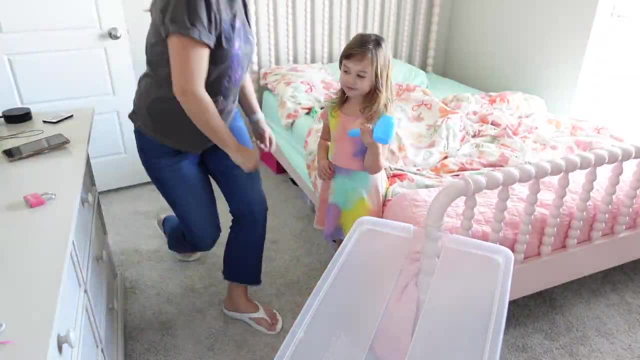 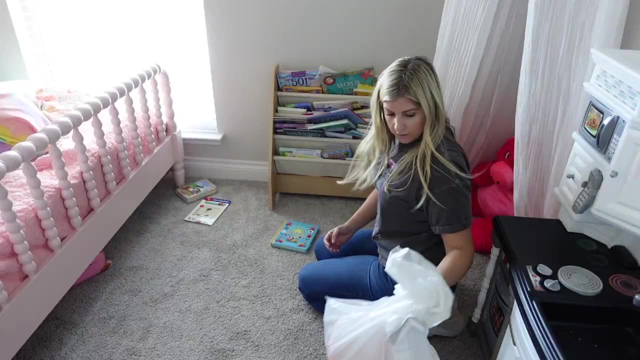 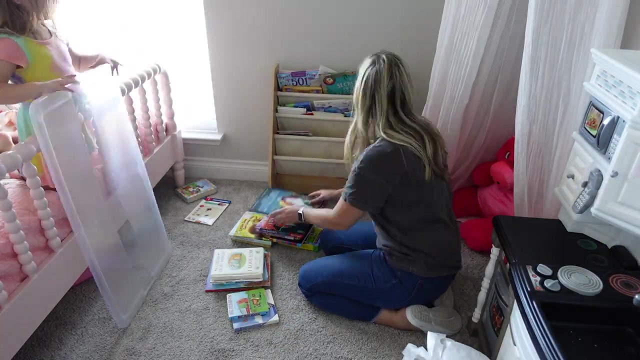 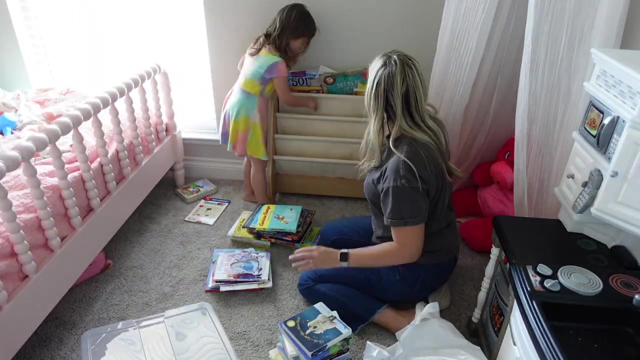 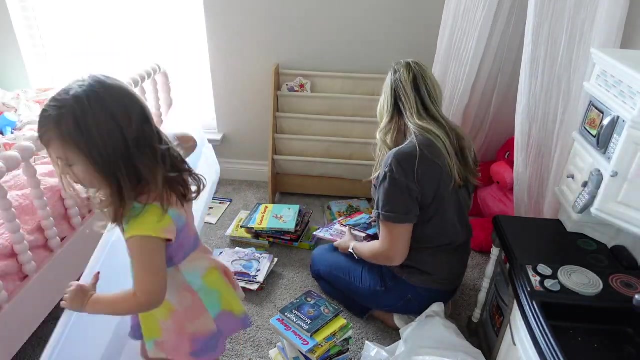 Cause we will still be high when the lights out. We can pretend the time is still, Stay in the daydream, Chase the thrill, Make up the way as we go. Live for the moment. Lose control. Rent a car you can't afford. Put us on that we both know. 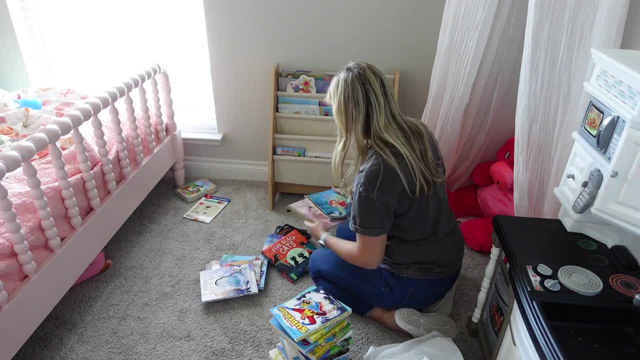 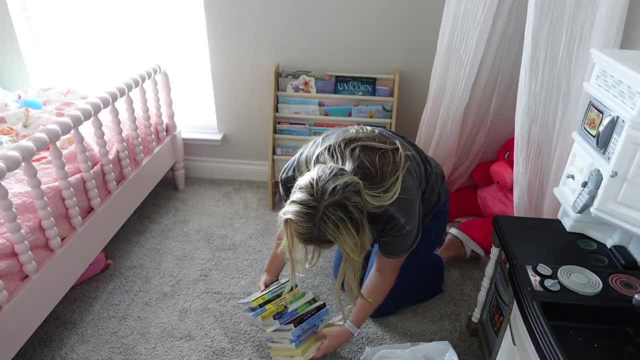 Let your hair out in the sun, Win. Put the pedal to the floor. Please tell me I'm not the only one with my kids' rooms in such a disastrous state. Comment down below and let me know if you feel the struggle of keeping your kids' room or playroom. 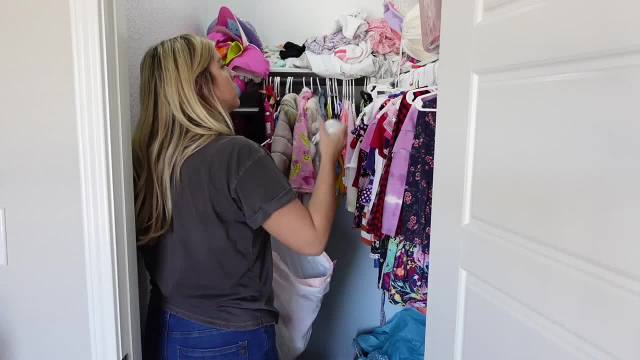 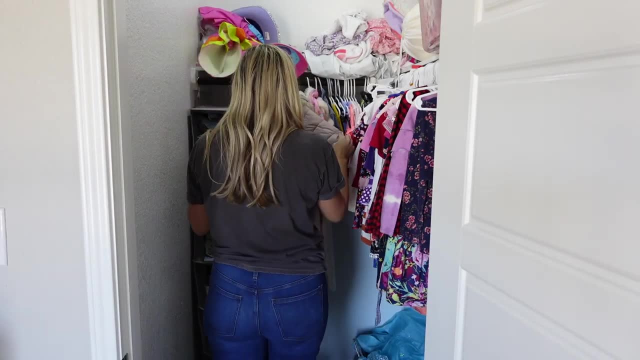 constantly organized. Brinley's closet is an absolute disaster in here And she has a lot of clothes that no longer fit her. So I'm sorting through items for keepsakes or to either hand down or donate. I'm also going to have a blanket made for her. I'm going to have a blanket made for her. 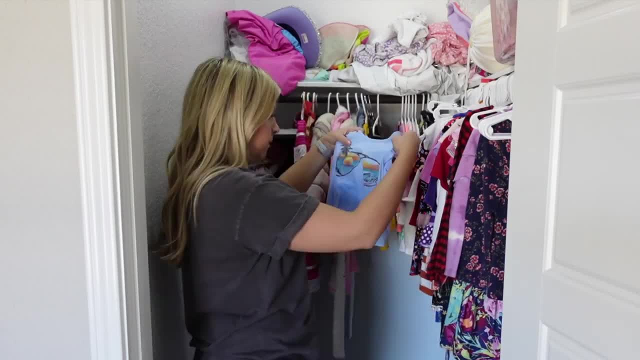 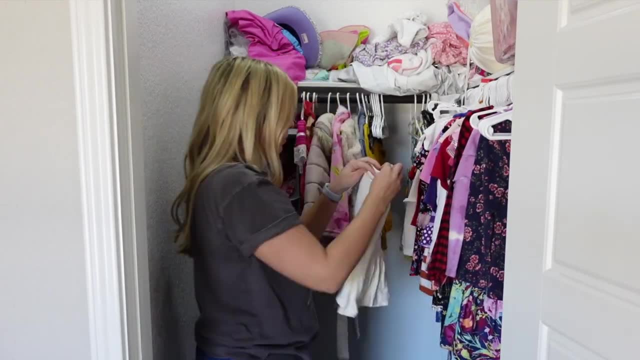 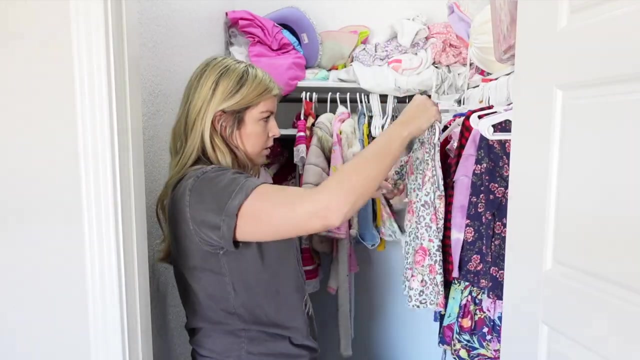 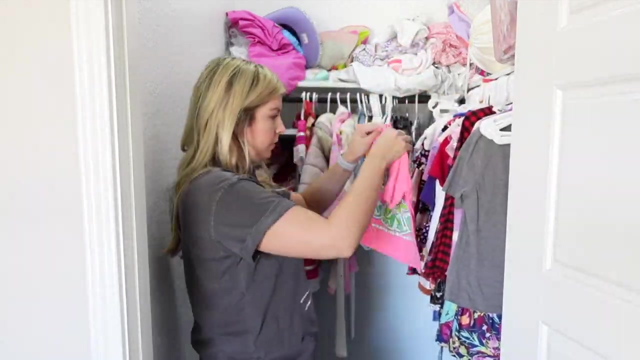 I'm going to have a blanket made for each of the kids with their baby clothes as keepsakes. Comment down below if you have done this. I'm really curious about it, Cause we will still be high when the lights out. We will still be high when the lights out. 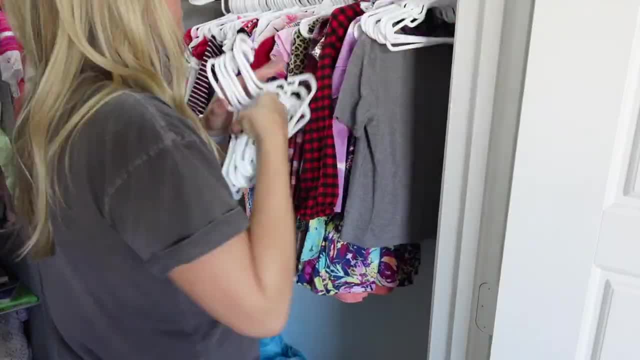 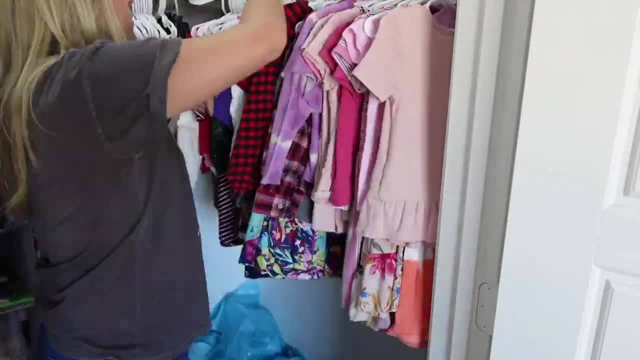 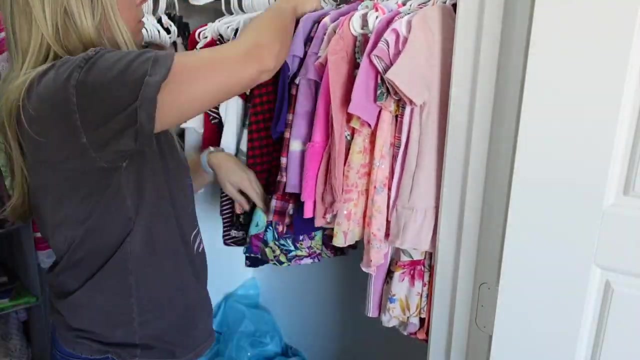 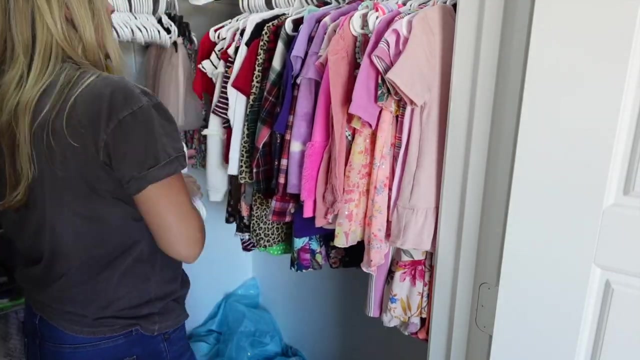 And if you tried, you wouldn't understand it. Maybe something's missing inside of you. Just a bit of sugar to that horrid bitter. Maybe you taste different. Hold up, hold up, baby. I can't sit beside you While you're going on about your simple life. 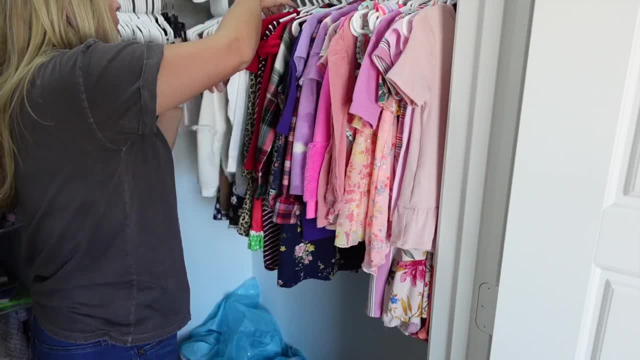 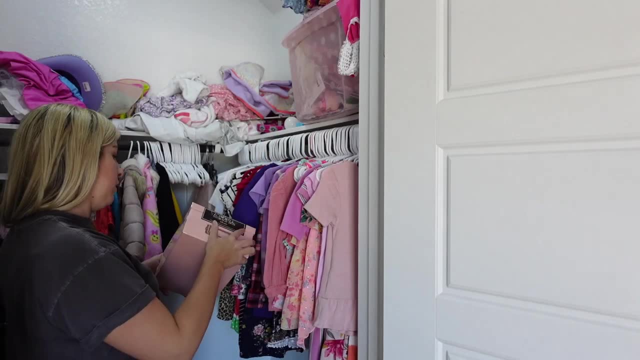 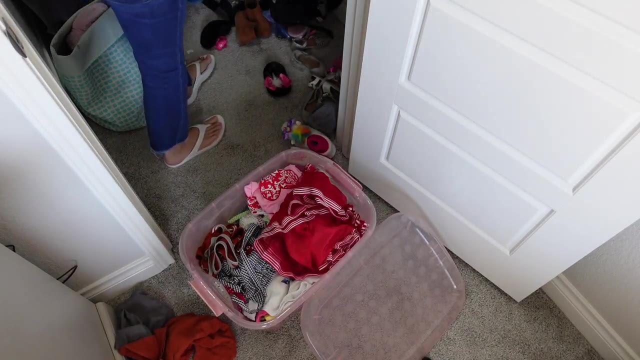 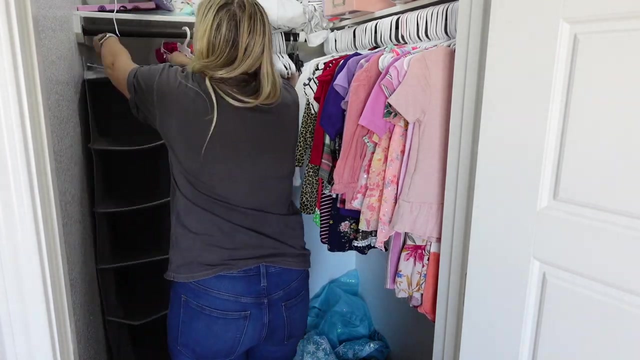 Nothing left. you're thinking that maybe you're not different? Go on, block your ego, Your ego, Your undenying, undying ego. Oh look, here he goes, Stepping on toes With his humble, lacking, everlasting ego. Oh look, here he goes. 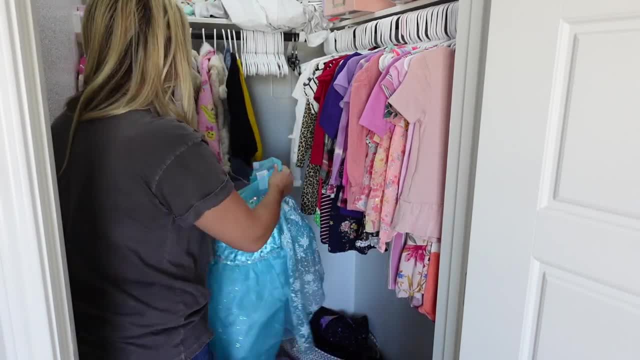 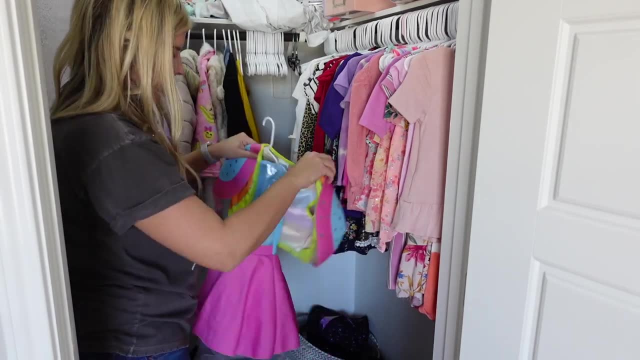 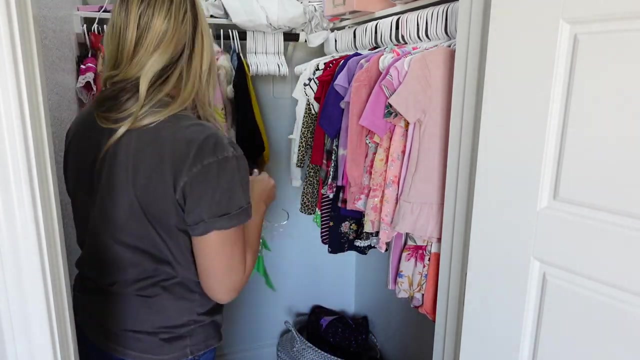 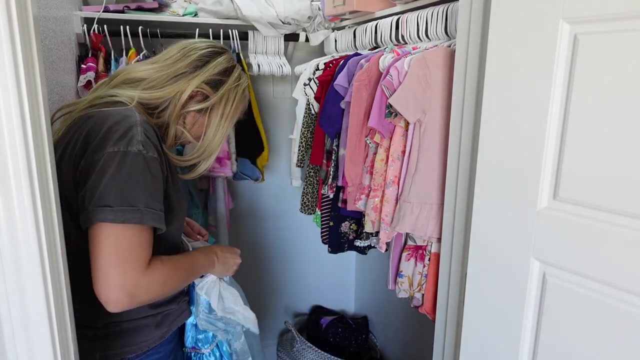 I guess it never hit you. Our conversation takes two, Paying it some interest from time to time. Inside all that greatness, In all of your adventures, You're all alone. Hold up, hold up, baby. I can't sit beside you While you're going on about your simple life. 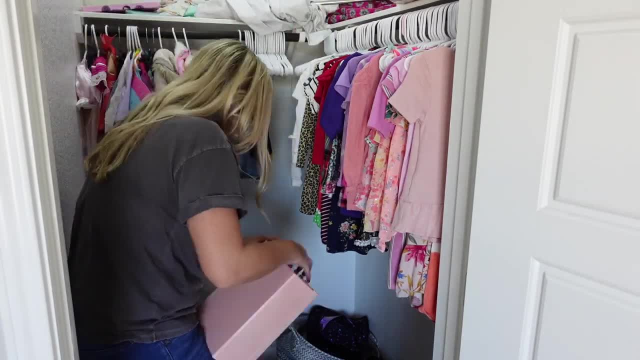 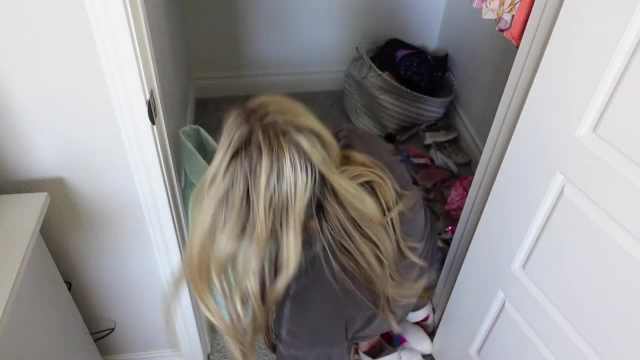 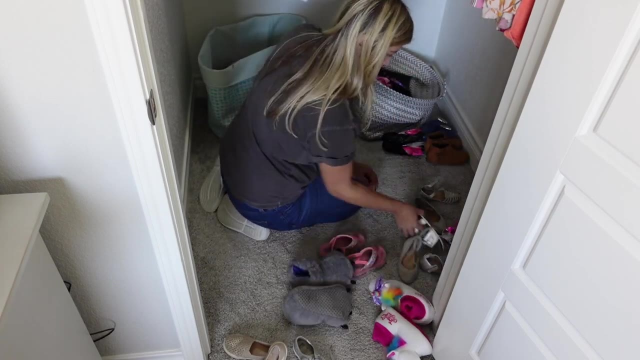 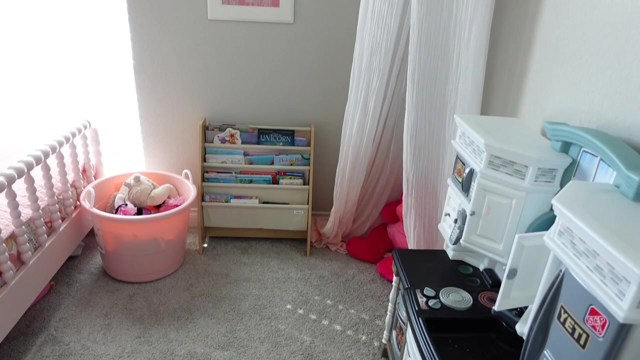 Nothing left. you're thinking that maybe you're not different? Go on, block your ego, Your undenying, undying ego. Oh look, here he goes, Stepping on toes With his humble, lacking, everlasting ego. Oh look, here he goes, Stepping on toes. 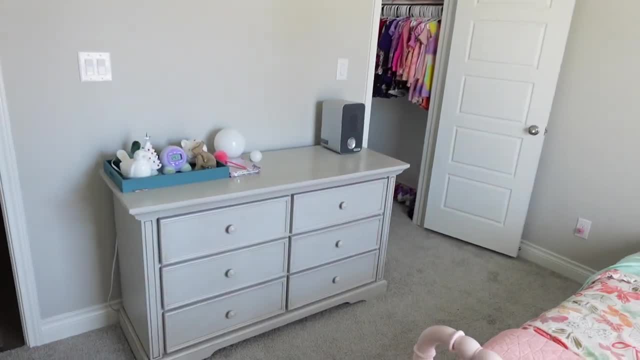 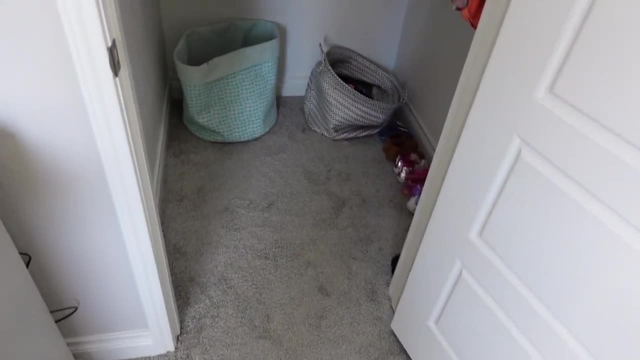 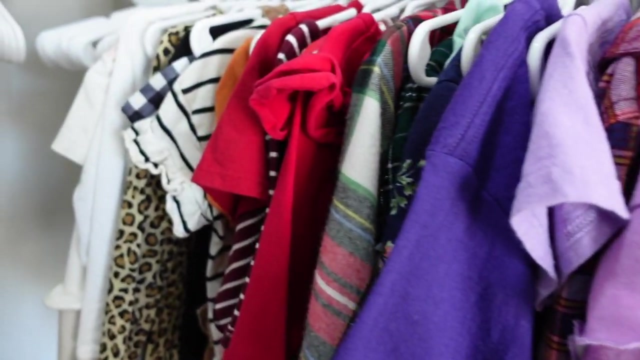 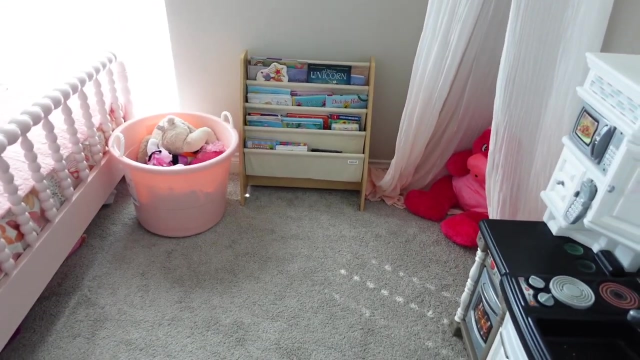 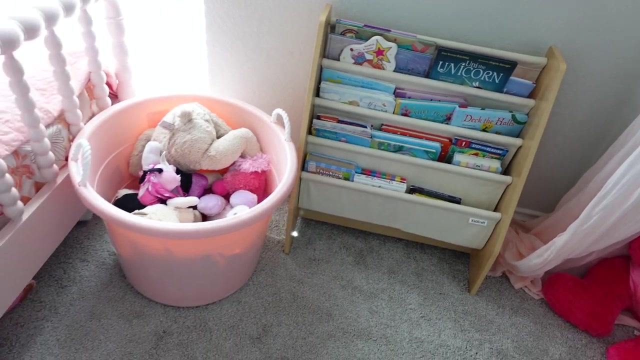 where these humble lacking ever last and he goes. oh, here he goes, here he goes, here he goes. such a huge difference. after decluttering and organizing brindley's room, i went through all of her books. she had a lot of books that we read to her as a baby and we're actually going to be. 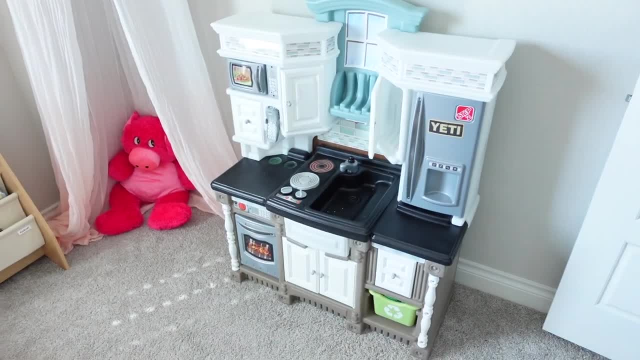 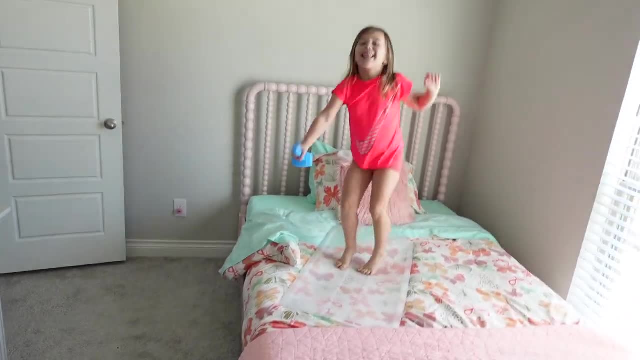 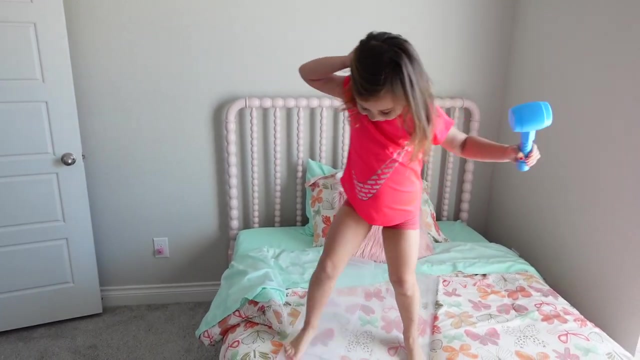 storing those away. i just cannot get rid of those. this kitchen set i will be storing in a different closet in the house. we are going to be doing a kids room makeover for both kids for part of their christmas. i'm so excited and i cannot wait to see the end result.